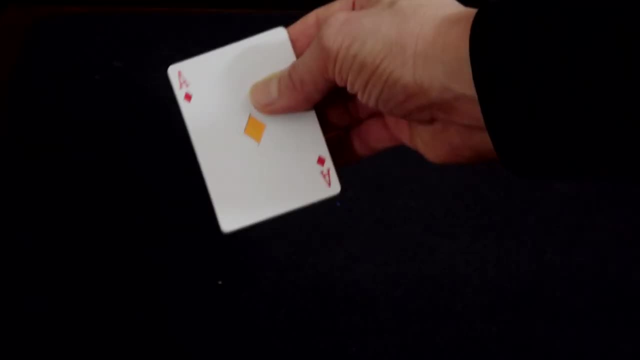 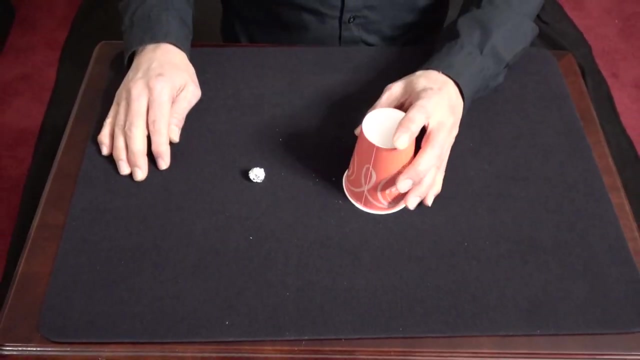 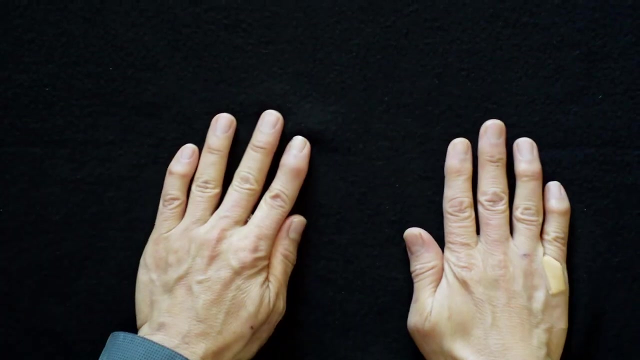 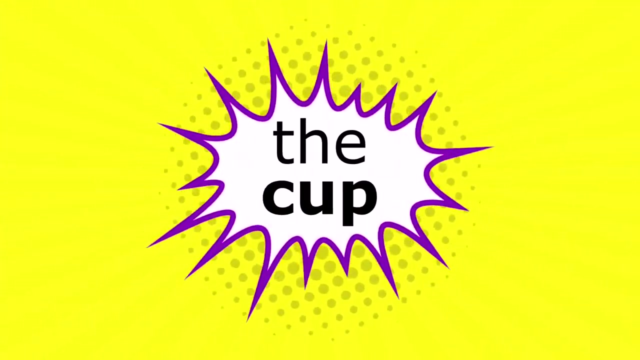 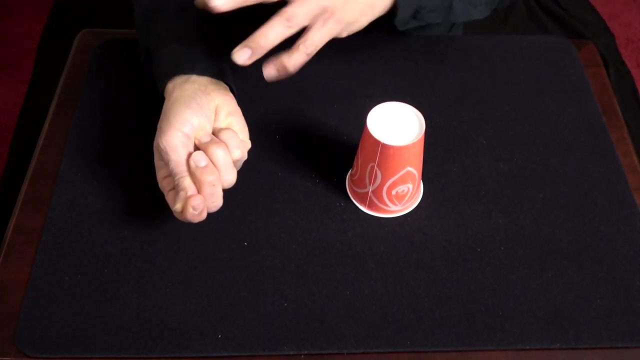 If you'd like to learn magic, we have 7 easy magic tricks that you can learn to fool your family and friends. Let's get started. Nothing here, A ball. Check this out, Wave the hand. The ball is gone. Where'd it go? 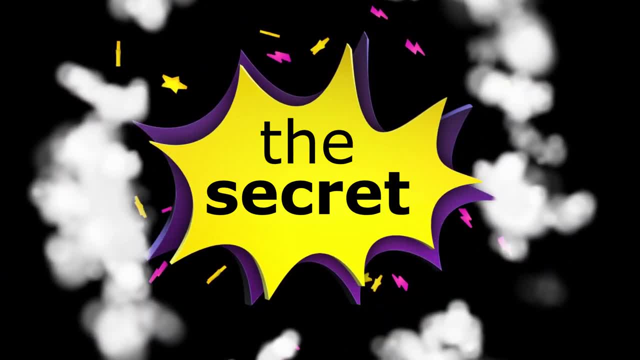 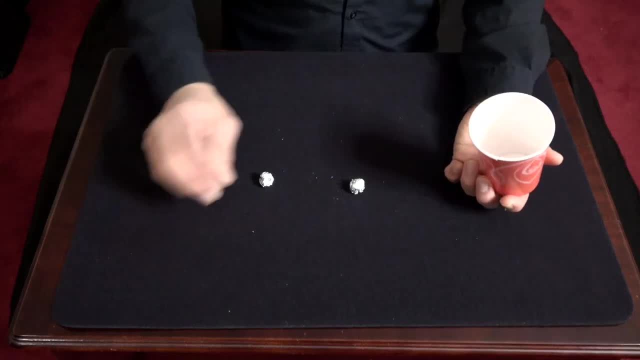 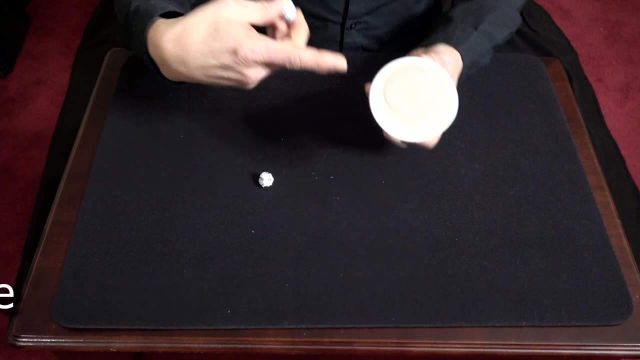 It's right, here under the cup, You're going to need two balls. Make them out of aluminum foil. just crumple them up Now. the cup has a piece of double stick tape at the bottom. Attach the ball to the cup. 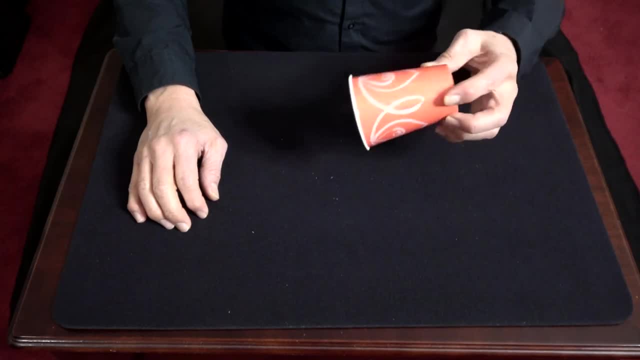 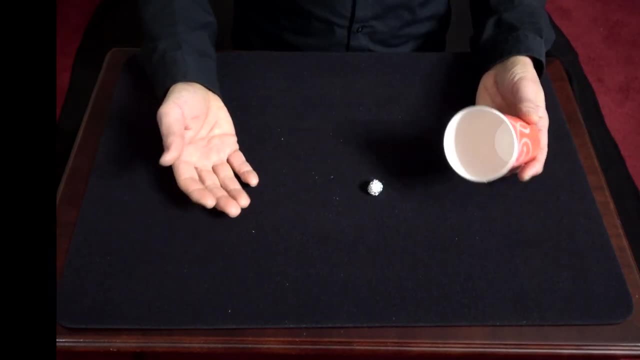 Attach the ball to the cup. Attach the ball to the cup: the double stick tape. Now that you've done this, you can show the cup empty, but when you drop it on the table, the ball appears. That's part one. let's get to the 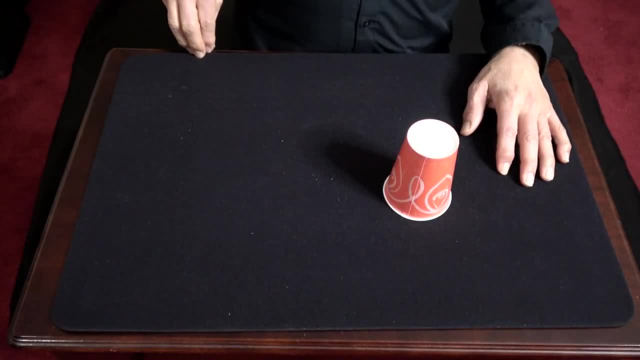 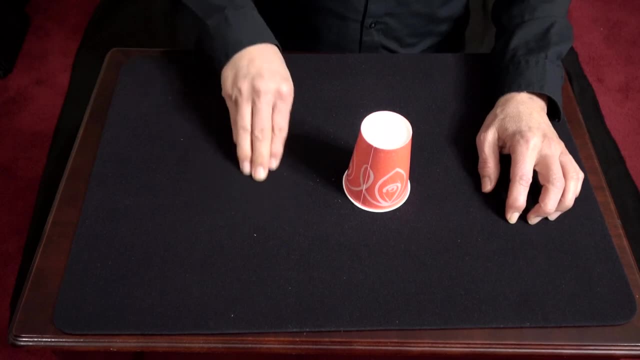 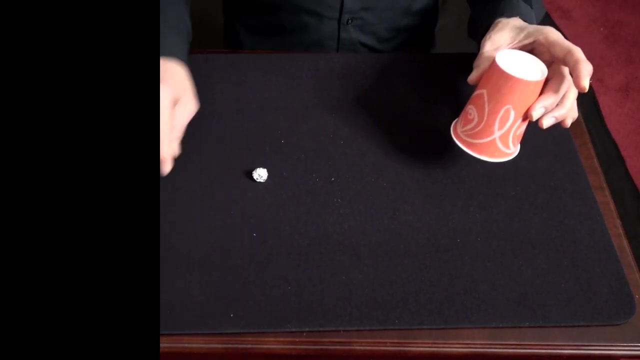 second part. When you grab the ball, you bring it to the edge of the table to pick it up, but what you're doing is actually secretly dropping it into your lap or on the floor. This is what it looks like. Now let's put it all together. 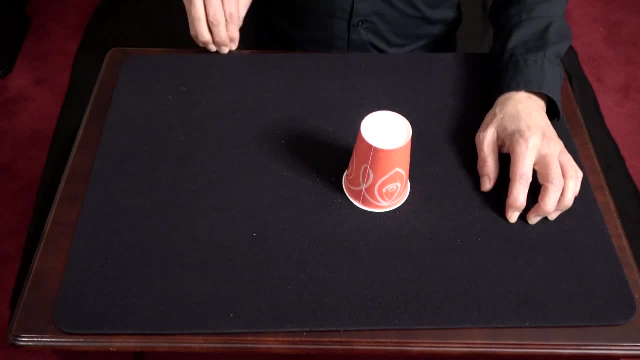 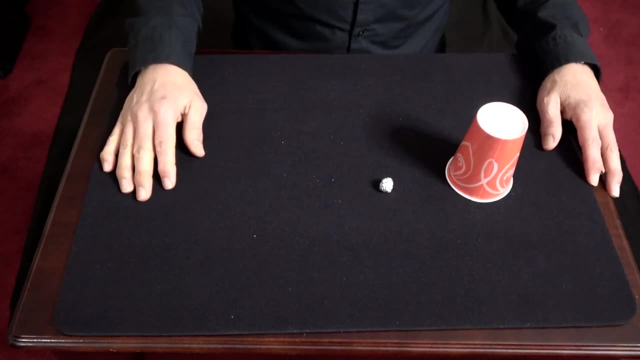 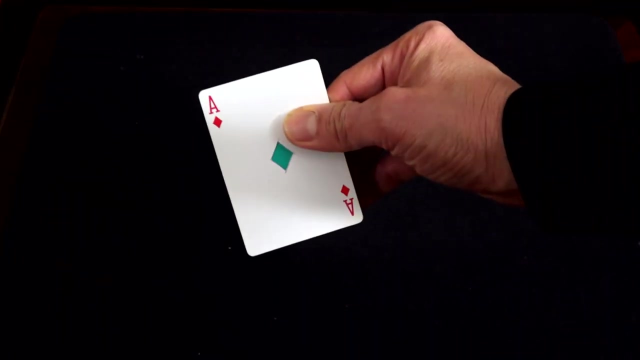 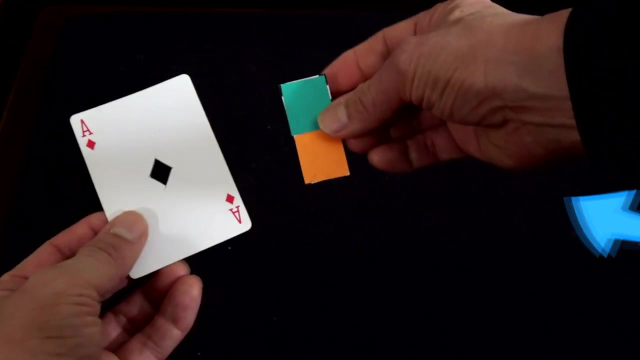 Nothing here. Grab the ball, drop it on the floor, Wave the hand Gone. Where is it Right? here? You're gonna have fun with this one. It's red, now it's blue. Here's the secret: You're gonna get an ace of diamonds. You're gonna cut out the. 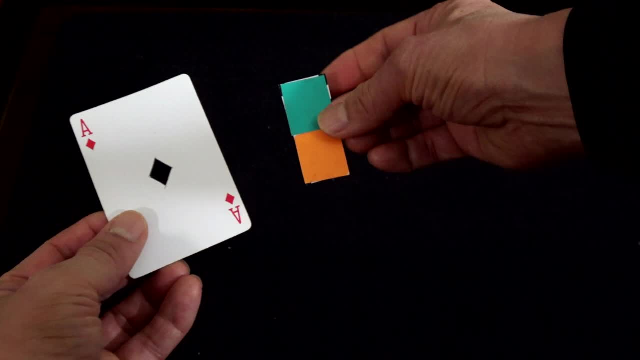 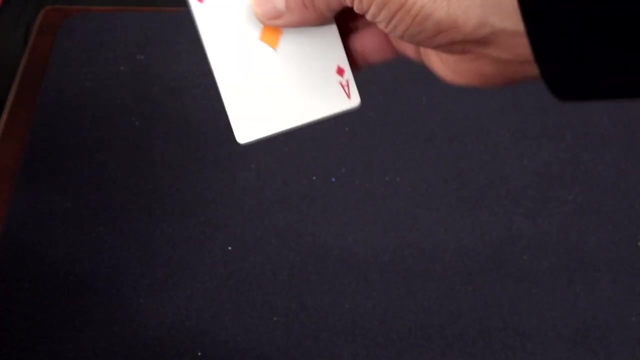 diamond, You're gonna need what I call a change card. It's just a little piece of cardboard. I use part of a playing card, Part of it's blue, Part of it's orange. Just position one color on the diamond and by moving your fingers you can. 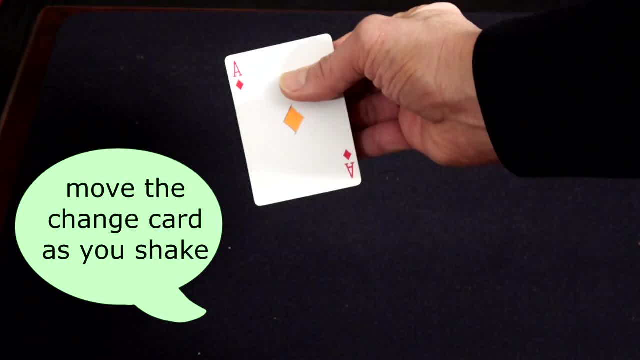 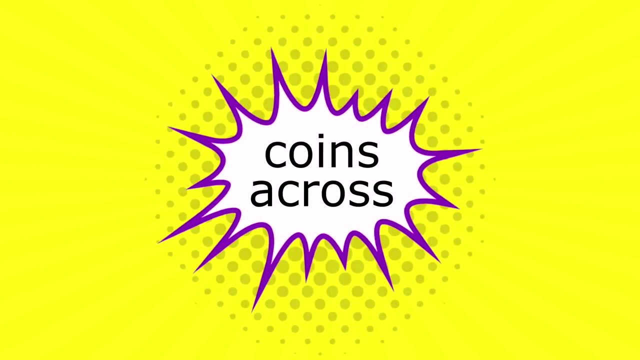 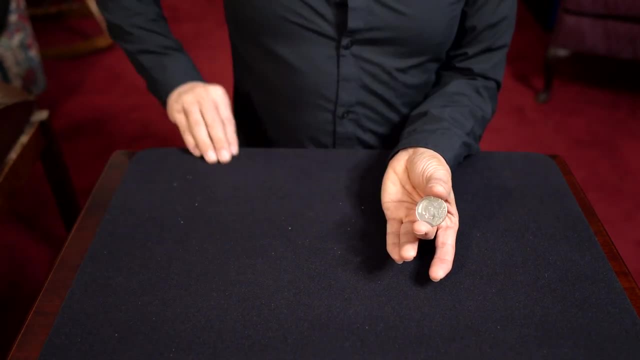 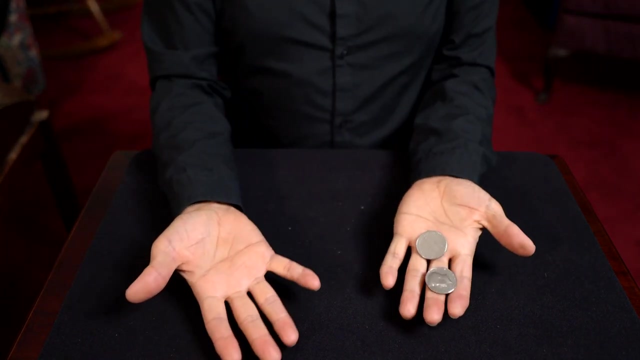 change the color. Now, to make it work Magic, Just shake your hand, Move your fingers and cause the card to change colors. Here's a cool coin trick. Here's a coin, Two coins actually. Check it out. I toss it. It goes invisible and joins the other coin in the other hand. You're. 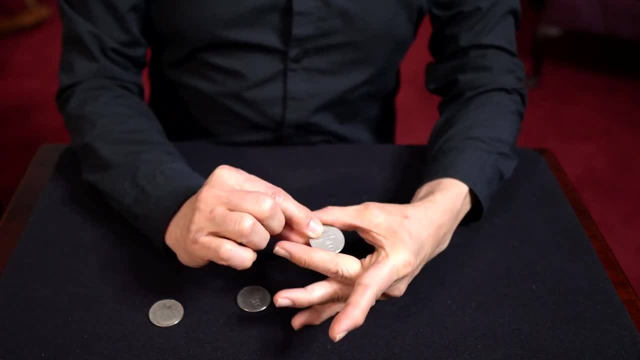 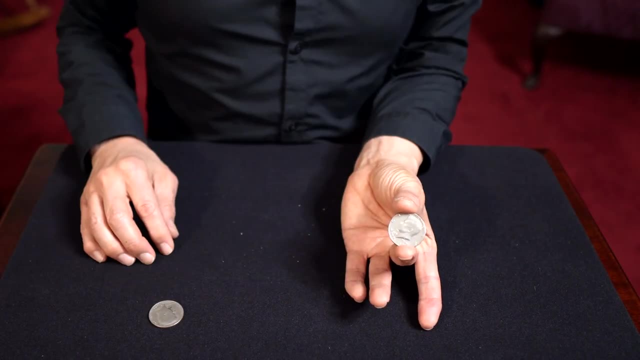 gonna need three coins. Here's the secret, though: You're gonna grab the coin and hold it in this odd kind of grip here. Now, when you take a second coin and place it in front, you can't see the first coin, and that's the. 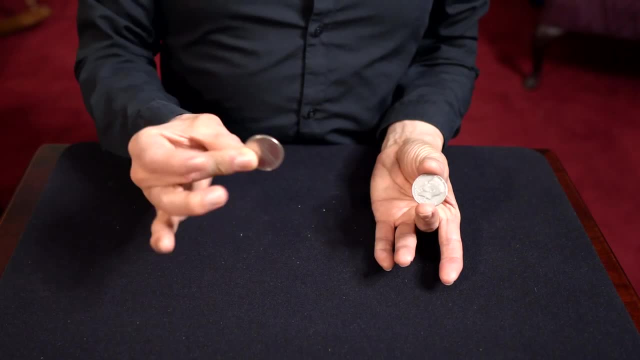 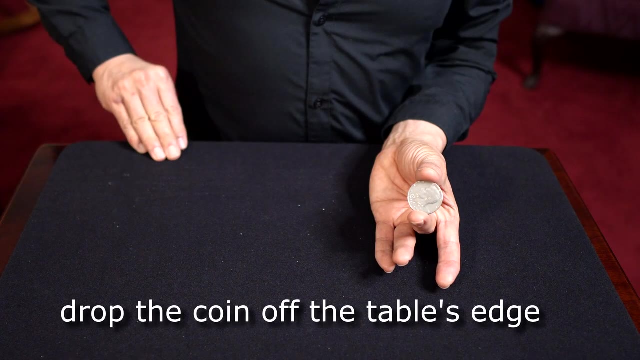 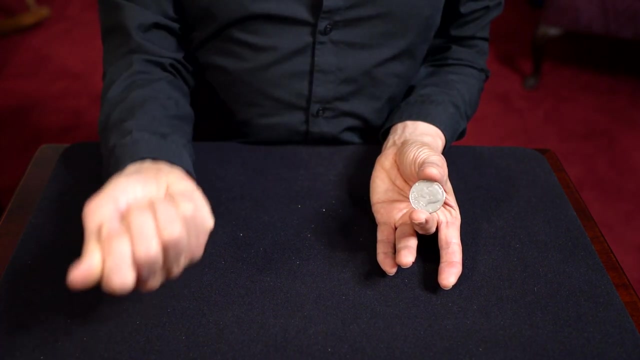 secret. You're actually secretly holding two coins. Now, just as we did in the earlier trick, you have to make the second or a third coin disappear. You're gonna drag to the edge of the table and once again, at that crucial moment, at the edge of the table, you let it drop into your lap or onto the floor. Your hand is. 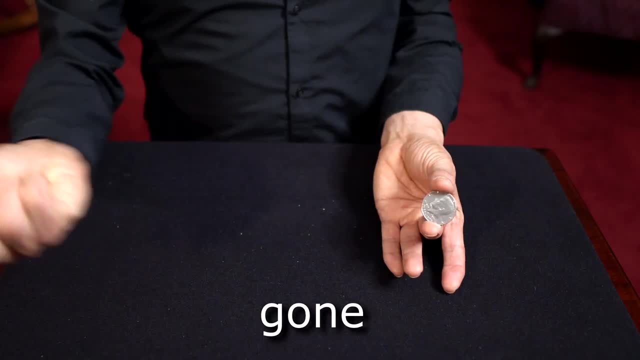 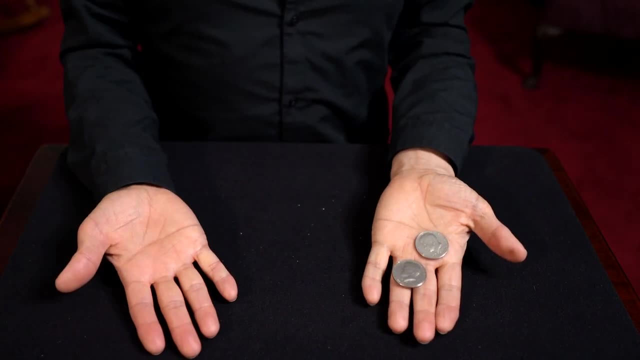 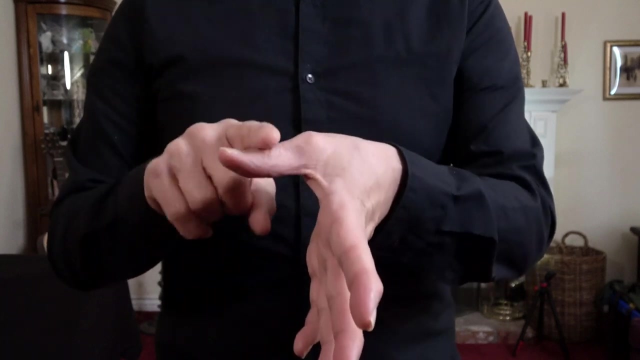 actually empty at this point. Now a little magic: Make the coin disappear and then let go of the coins and they appear in your hand. Here's a trick that every uncle and grandpa has to know: The thumb trick. I'm gonna teach you how to do this. 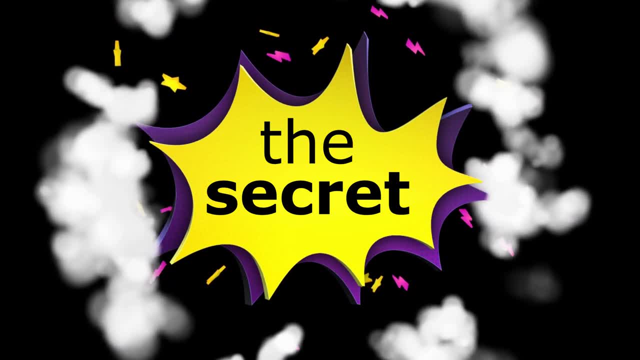 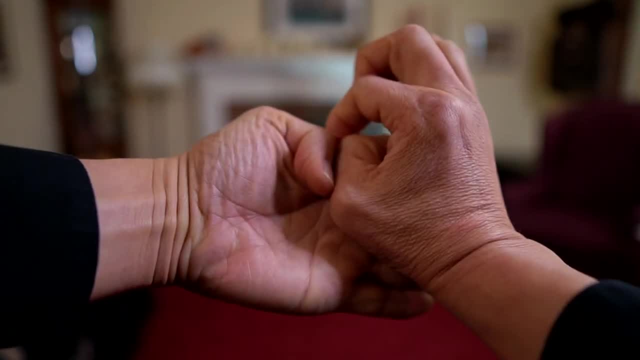 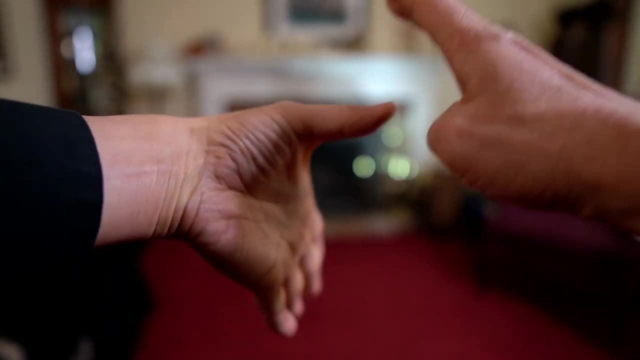 You can do this anywhere, anytime. All you need are your hands. You're gonna position your thumbs in the following way, and your finger goes over the in-between part, So it looks as if you're splitting your thumb. Now you have to get into it. I like. 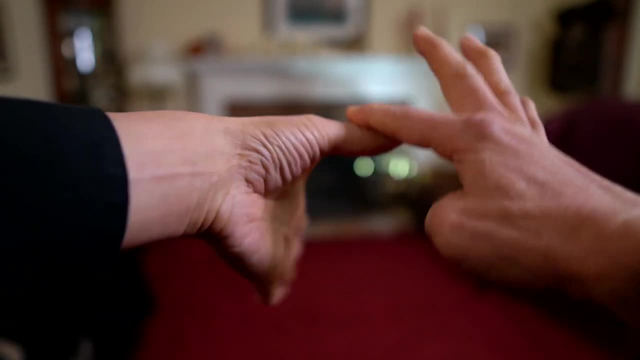 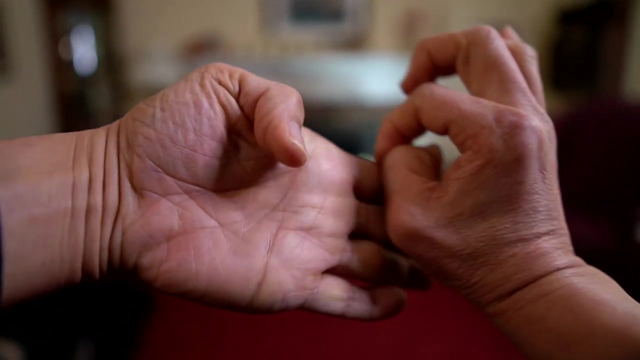 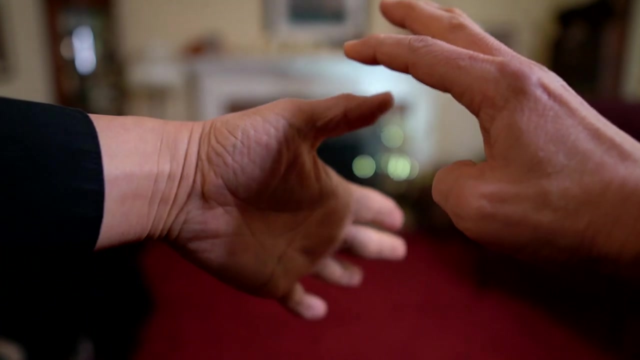 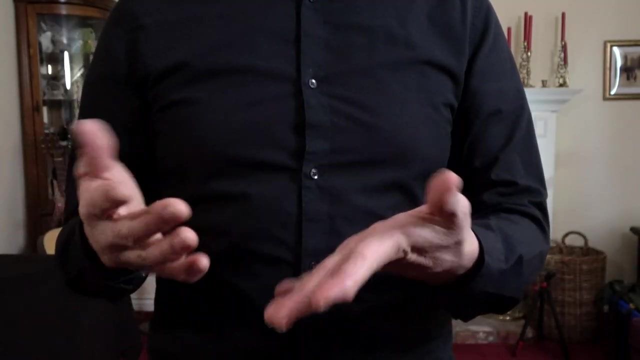 to tap with my index finger and then move my thumbs in. Do it slowly. You have to learn to do this quickly. So here we go in just real time. I kind of feel like I'm gonna do it for the kids. You can see, I'm going and I'm. 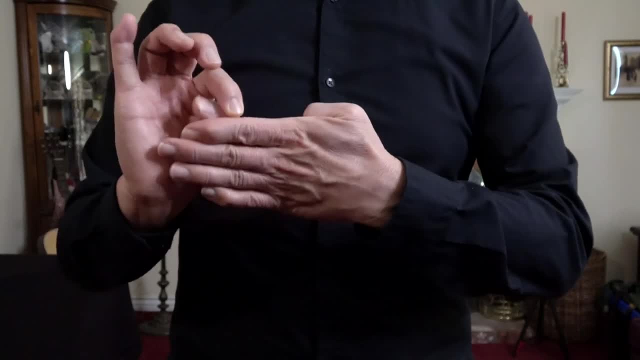 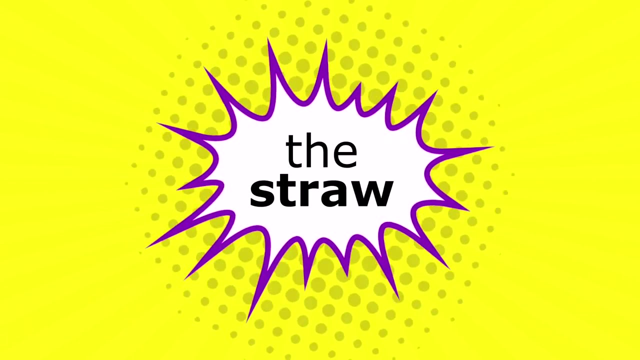 gonna tap and do the magic trick. There we go. So You can see, theуки is pretty fast. You can see the cloud: I'm gonna tap, use your fingers. You can see the moon: I'm gonna tap and you're gonna tap your fingers. 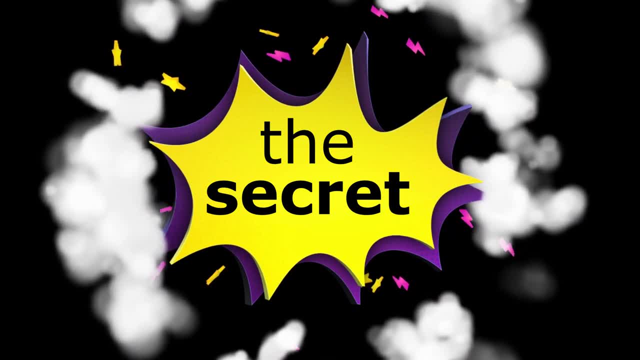 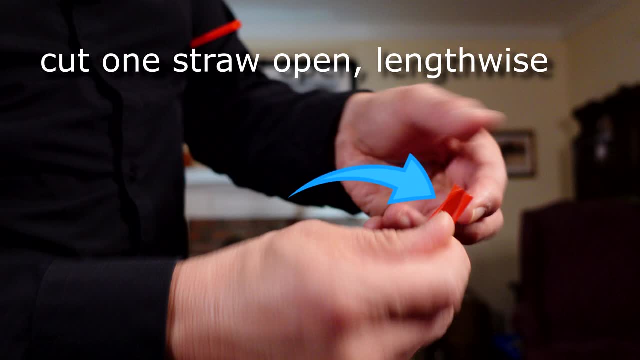 Now this is going to be a little bit faster. It has to be that fast, And now, from the regular view, you can see how fast it is. Now you know the secret and you could perform this for the kids. Take the first one and, using some scissors, cut it all the way down the length of the straw. 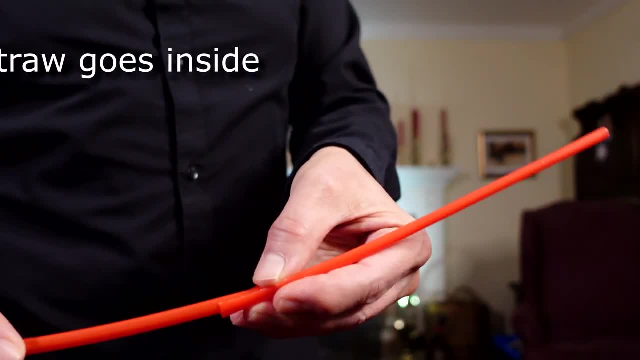 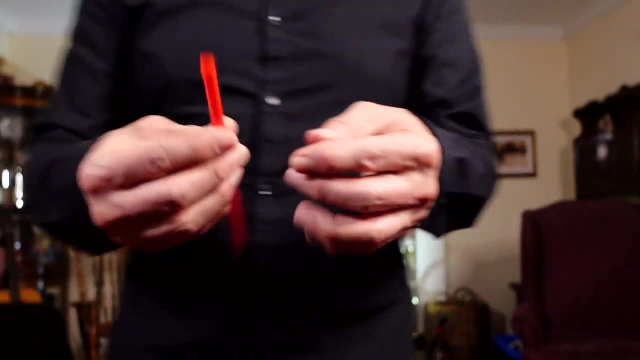 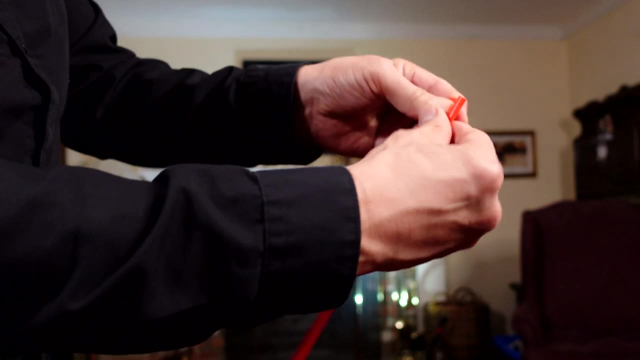 Take a second straw, feed it into the first straw. Now it appears that you have a single straw. Just handle it, show it to the audience and then, when you're ready to produce the second straw, you pull the second one out and it looks as if you've magically split the single straw. 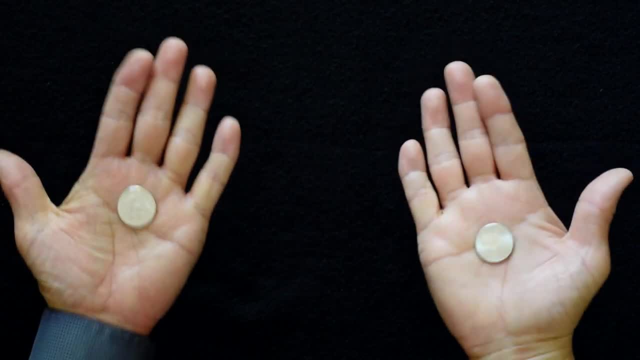 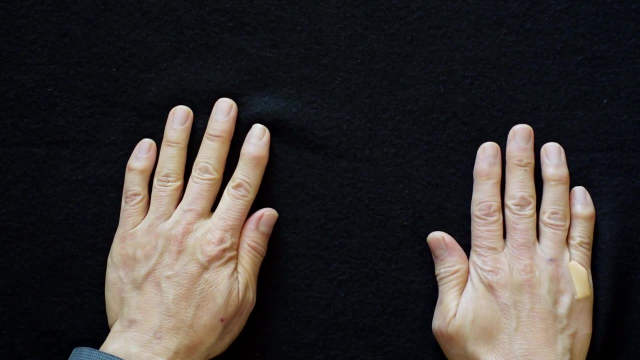 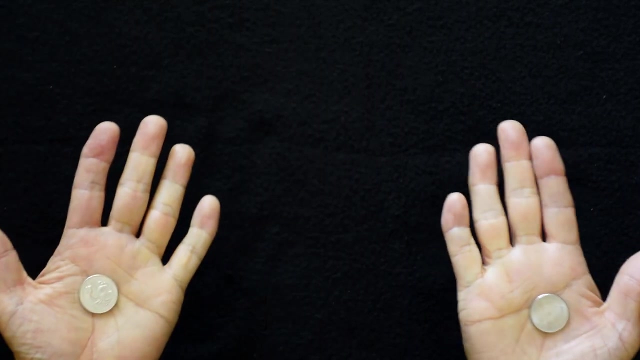 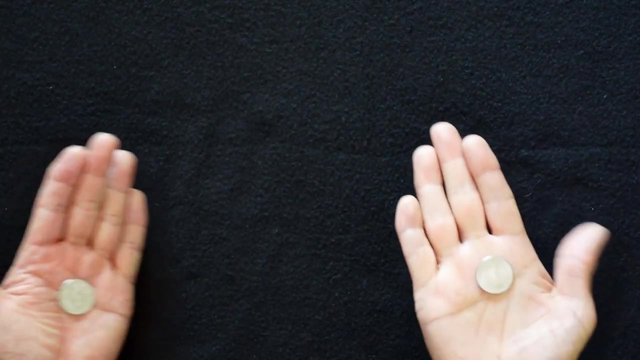 Here's another trick with coins: Two coins, one in each hand, and they join each other. This is a fast trick and all you need are two coins, One coin in each hand. You're essentially just tossing one coin individually. Then you turn the coin to the other hand as you turn the hands. 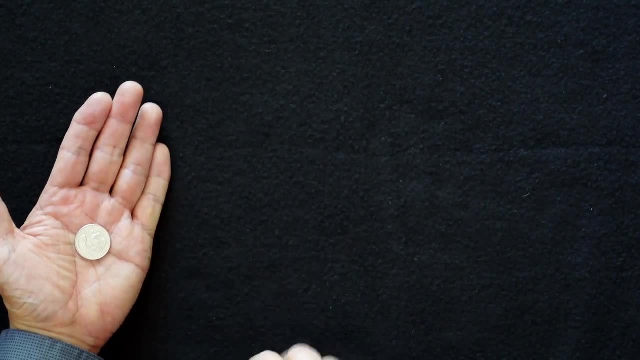 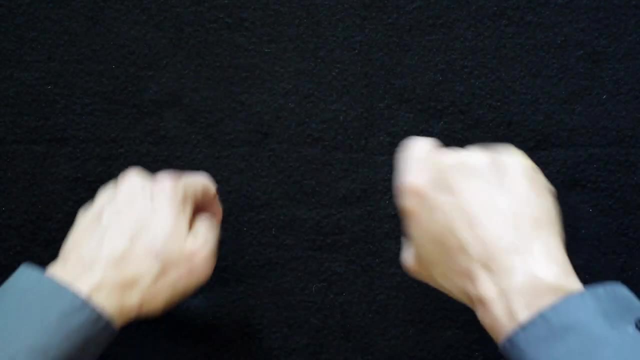 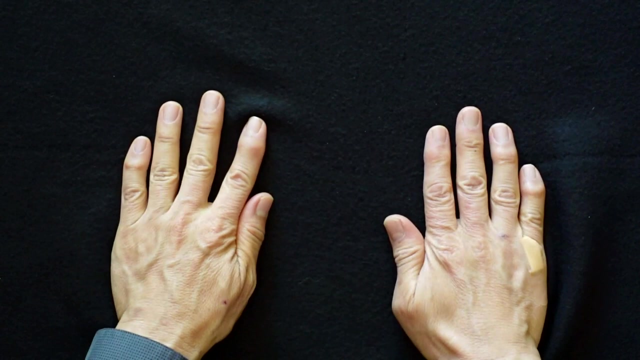 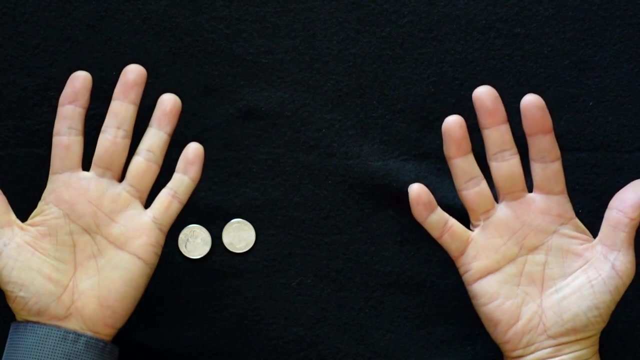 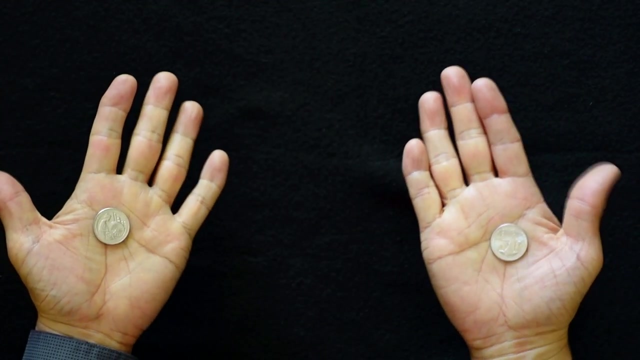 As you can see, it has to be a really fast motion. There you go, See how fast you have to do it, And the second hand turns over and catches the other coin. Let's show this to you in slow motion And I think you'll see, even under slow motion it's pretty hard to catch. 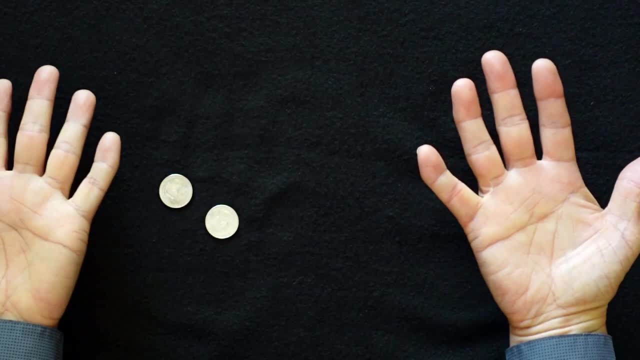 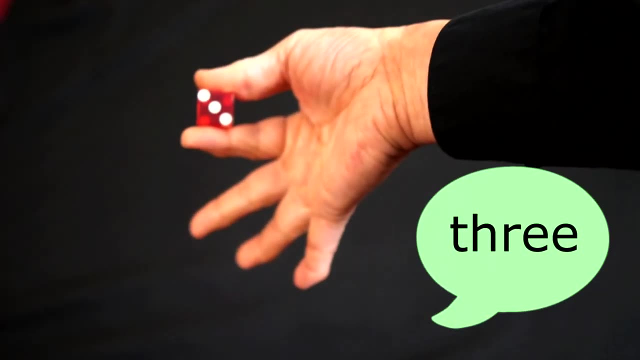 But you can just get a glimpse of that coin flying over. You'll have fun with this one. All you need is a table and two coins. Now, here's something for game night. If you have a die with you Now, I turn it over. 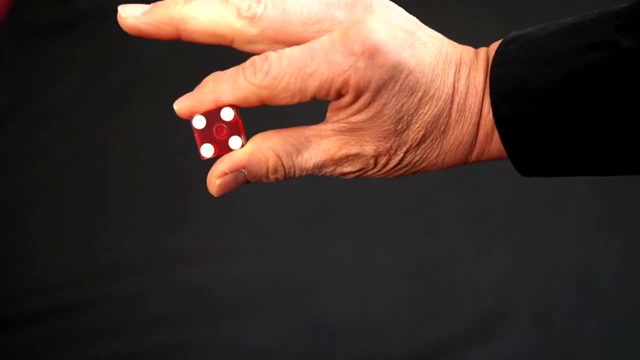 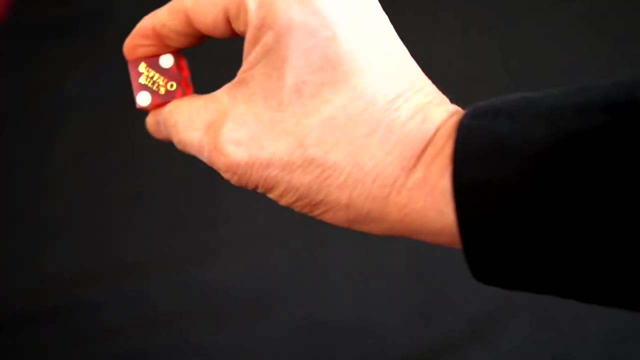 There's a four on this side, There is a three, on the other side Four And three, But magic, Now there's a two. All you're going to need to know is a secret move. Now I'm actually turning the die over here. 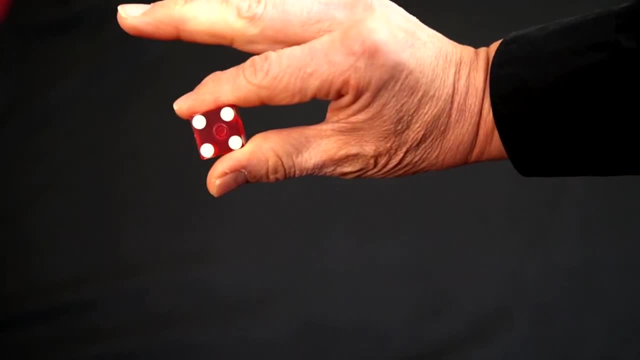 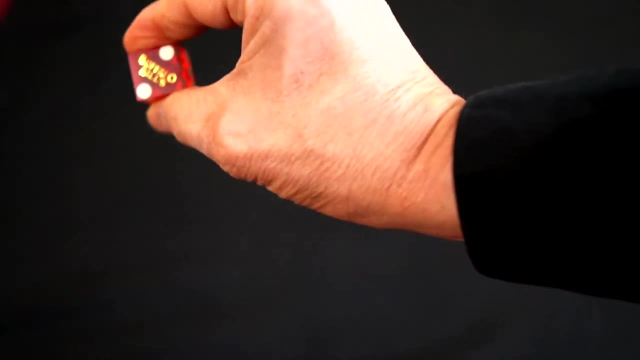 And it doesn't matter what numbers you use, But on the third time I do the magic move. I'm going to turn this over, And I'm going to turn this over, And I'm going to turn this over, And I'm going to turn this over.